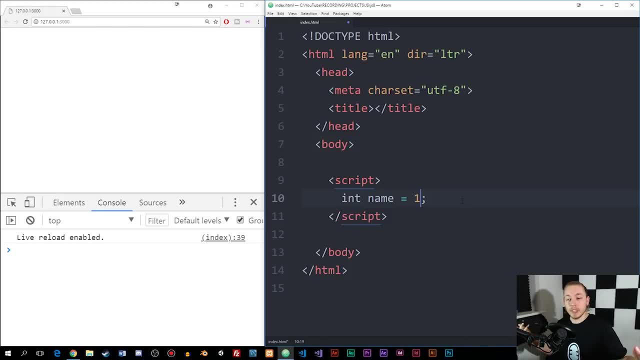 some kind of number, because that's a number, an integer. So in JavaScript we just use the keyword called var in order to define that we have a variable. And this is going to be relevant a little bit later on in this lesson when I start talking about how we can actually figure out what. 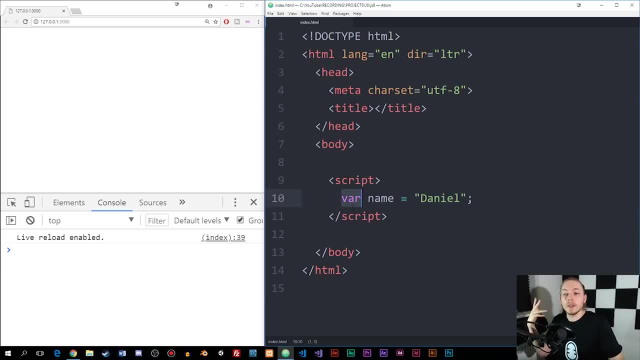 kind of data we have inside a variable, because right now we can't really see what kind of data we have inside this specific variable. So let's say that we have a variable that is inside this variable Other than looking at the data, which is right here, but when we look at it inside the browser, 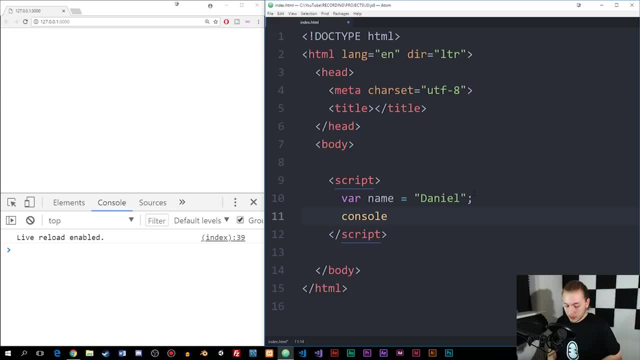 if we were to actually console log what we have here- consolelog parentheses- and then put this variable and log it inside my console. inside the browser you're actually going to notice that we just have Daniel, But I can't tell what kind of data this is, even though I could probably guess. 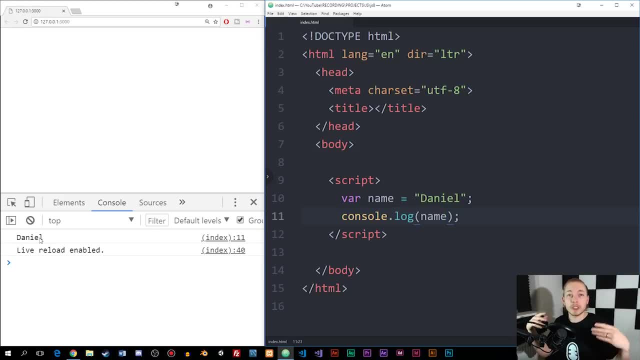 this is going to be a string, because it has characters and it's a word, but we can't really tell By looking at the browser here what exactly this type of variable is. So later on in this episode I'm going to go and show you how we can figure that out, But before then we're just going to go. 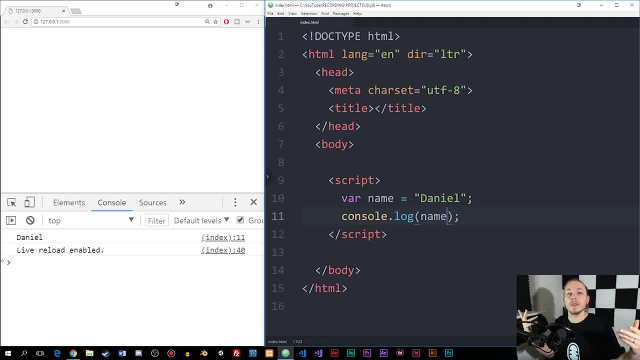 and talk about the different types of variables that we have, or not different types of variables, but different types of data we have inside JavaScript. Now, the first data type that I want to talk about in this episode is something called the string data type, And I did just create an. 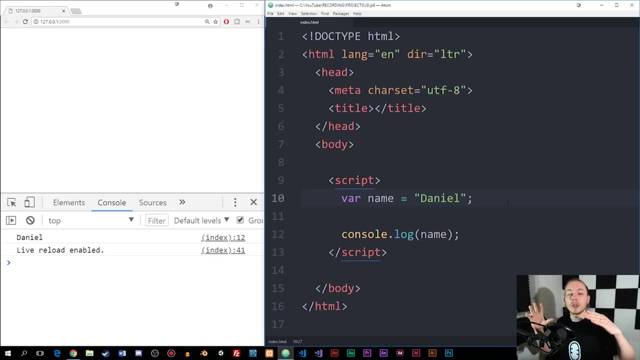 example of it right here. And a string is: essentially, we create a word or sentence using characters. Now we can define a string by wrapping double quotes around whatever word we want to create, And it's very important that when you create text, you need to make sure you wrap the text inside double 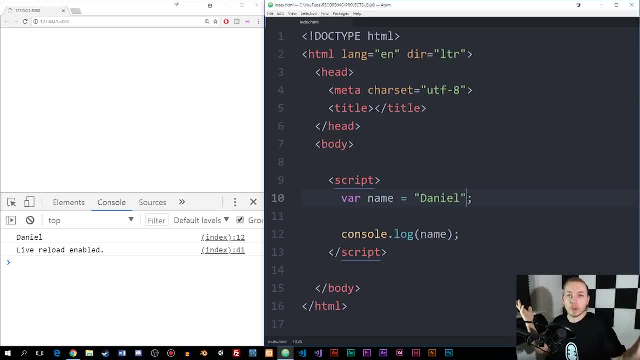 quotes, Otherwise it's not going to be seen as a string, which is what we call text. So if we were to remove these double quotes and save it, you can now see we get a uncut reference error inside the browser because it doesn't know what Daniel is defined as. what kind of data is Daniel? So we 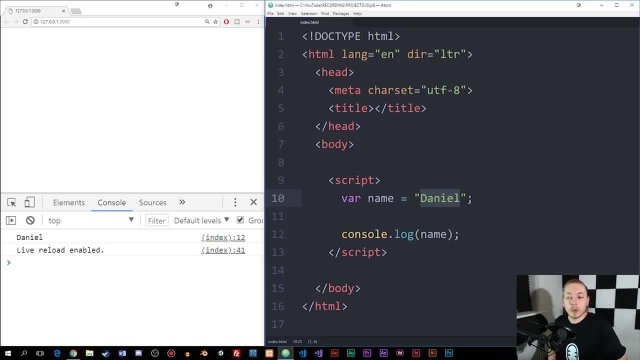 need to make sure that we go ahead and wrap double quotes around the data here. Now we could also go ahead and use single quotes, So we could just use single quote like. so it's also going to work. Now there's not really a big difference between using double. 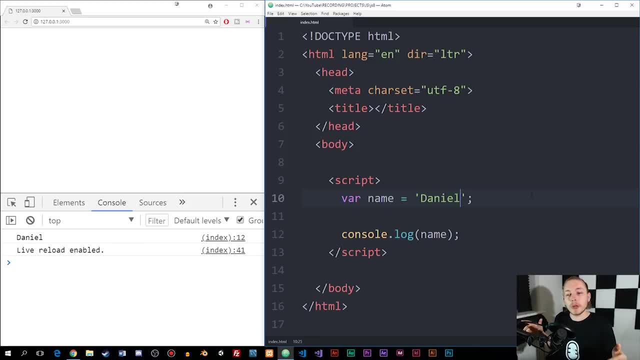 quotes and single quotes when it comes to JavaScript, but when we create a string using, for example, single quotes and want to write some text inside of it, If I say, Daniel is Nilsen, because that's my ealt name, if I can actually spell that out- 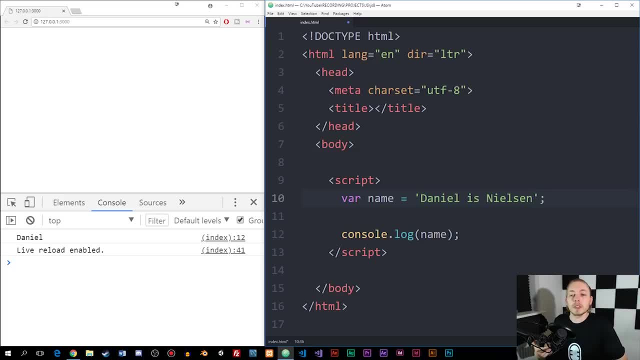 because that's my e las name, if I can actually spell that out, Or just to say: you respond to the process in your electronic documents that are stored inside your common folder. So I'm not makingkt correctly if I want to use double quotes inside the actual string as part of the 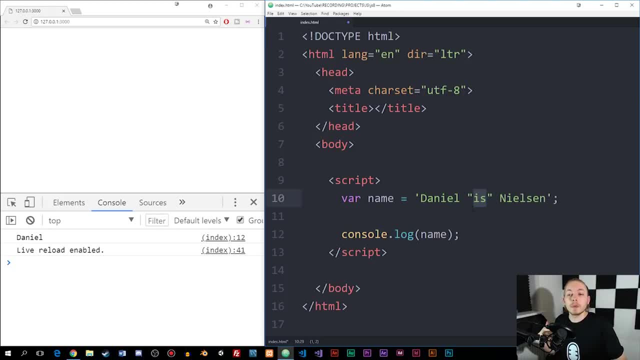 text that I need to make sure that I didn't use double quotes around the string, otherwise it's going to cancel out. I don't know if you could just hear my dog snoring is right underneath me, otherwise it's going to cancel out the string. and when I say that I mean that if it were to actually go here and do 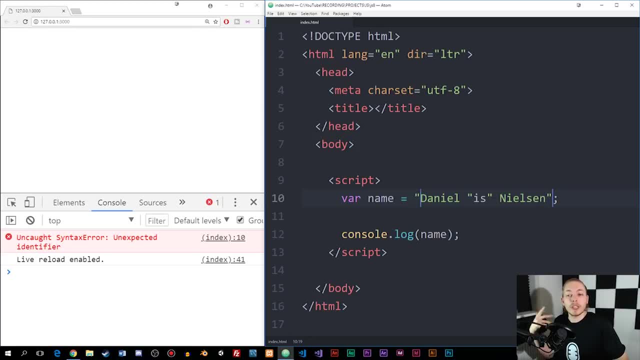 like this, where I'm using double quotes around the entire string and inside the string. then you can see that is has a different color and we get an error inside the browser because we just cancel out the string and continued it afterwards, which we can't really do. so in this example we could also say it's: 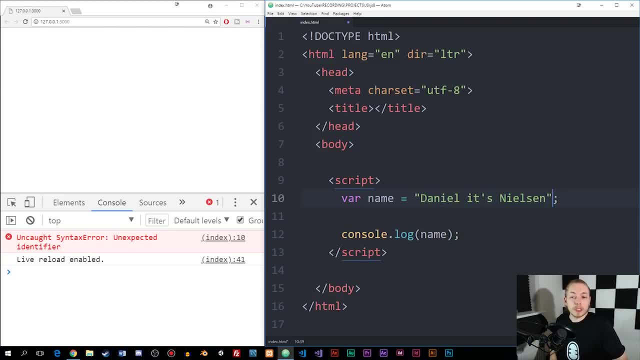 where use a single quote. in this example, the same thing goes. we can't use single quotes around it, otherwise it's going to give us an error. now I do want to show you another example of a double quote. because I'm using double quotes around double quotes. because I'm using double quotes around the entire string and inside. 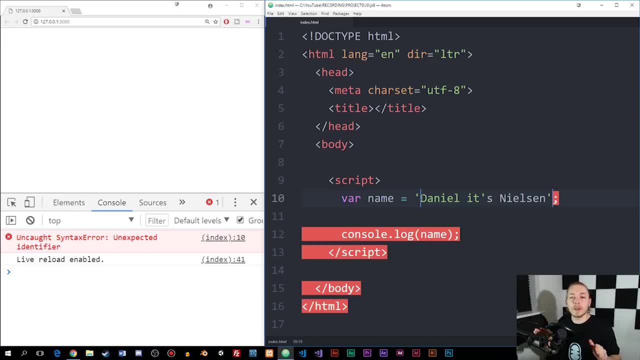 example here, because this might not be the best way of solving the issue. if you, let's say, you have a piece of text that has both double quotes and single quotes inside the actual text, then we can't really use the solution where we just switch out the quotes around the string. so in this case we would actually need 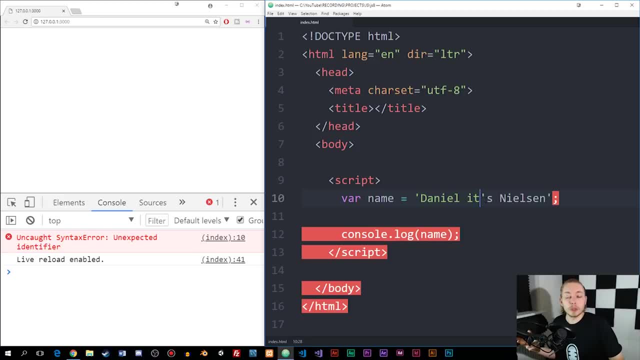 to escape the symbol or the character that we use inside the string. so if I'm using single quotes around the string and I want to use its as part of the string, then I need to escape the single quote inside the string, if that makes sense. so what I can do is I can write backslash right in front of the single. 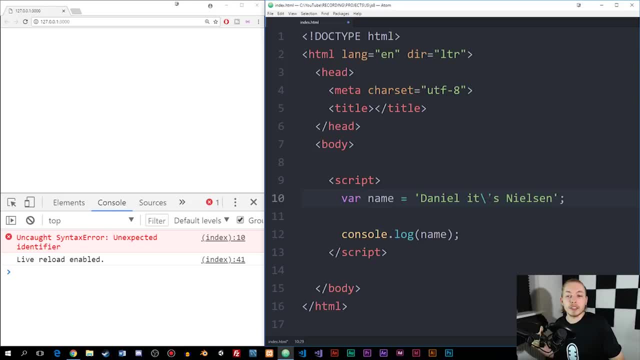 quote and now it's going to escape the single quote and not see it as part of, you know, defining a string. so if we were to save this, you can see that we still have the single quote inside the browser, but actually zoom in so you can see it. 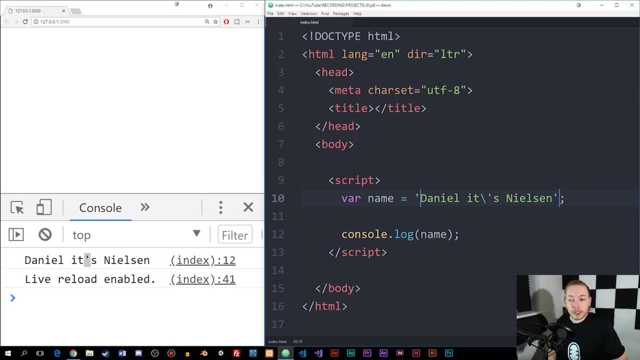 there we go. and the same thing goes if I were to go around the string and use double quotes. there we go, save it, and I can see we escape the characters inside the string. so this would be the best way of doing it if you were to use the string wrapping inside. 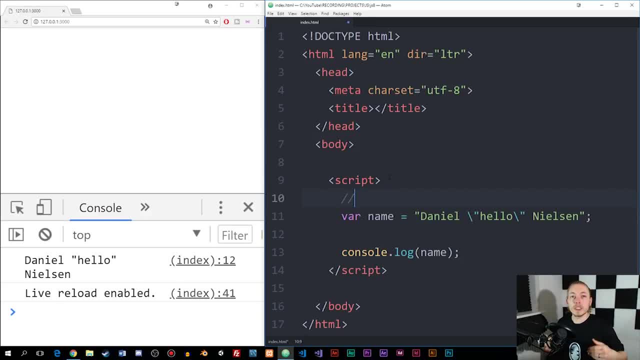 the actual string. now I'm just going to go ahead and create a comment here. so you know that this is a string data type. so I'm gonna write string data type. there we go, and then I'm gonna go ahead and go down to the next line. now what? 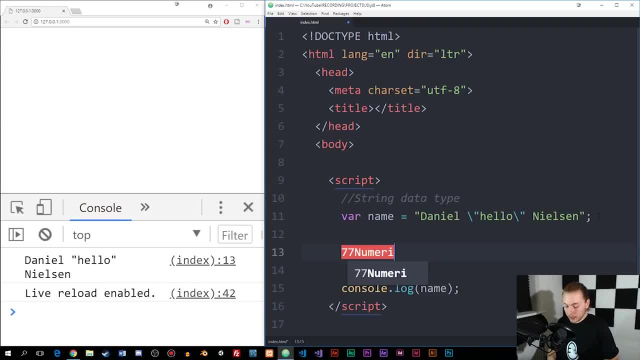 I'm gonna do is I'm gonna go ahead and create something called a numeric data type, which means numbers, and I did not write forward slashes. I need to make sure I do that. there we go now. a numeric data type is when we use numbers inside variables and we basically have two. 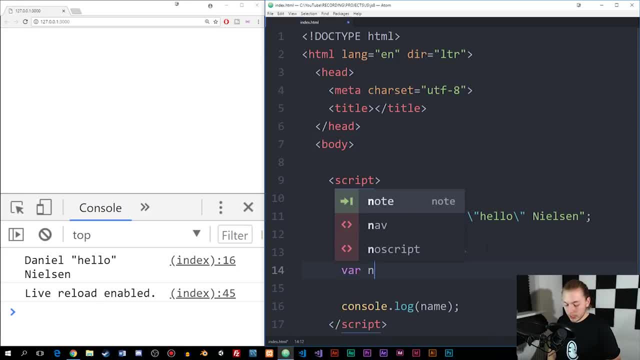 different types you can use. the first example here is going to be: I'm just gonna create a variable which I could just call num1, so the equal to 1, which will be a number type inside a variable. now we could also do like this, just to: 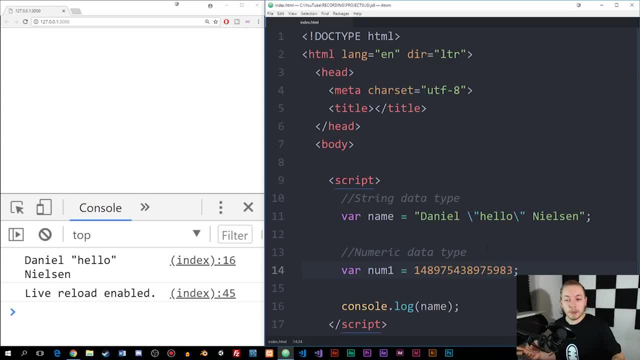 create something longer, and this is still going to be a number type. now we also have something called a number type, called a number type. now we also have a integer. Now an integer- if I just create another variable here, is going to be a number that has decimal points behind it. So if I were to say this, 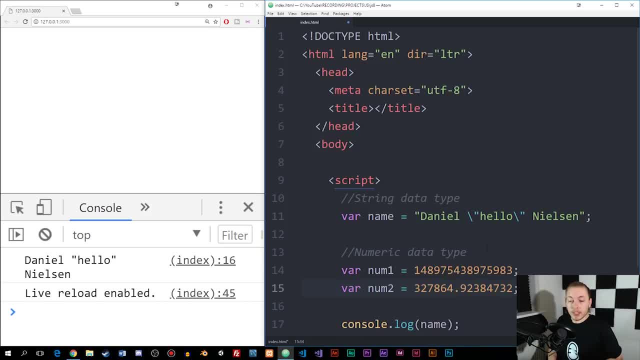 number here, dot, something- is going to be an integer, So it just has some kind of decimal points behind it. And the same goes for negative numbers. If I were to go inside num1, if I were to write negative, whatever number we have here, 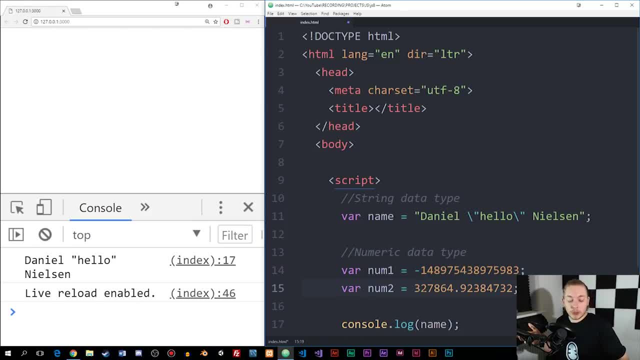 it's still going to be a number. And if I were to go down to next one here and do the same thing, it's still going to be an integer. So negatives and positives both go when it comes to number types. Now there's another thing I want to. 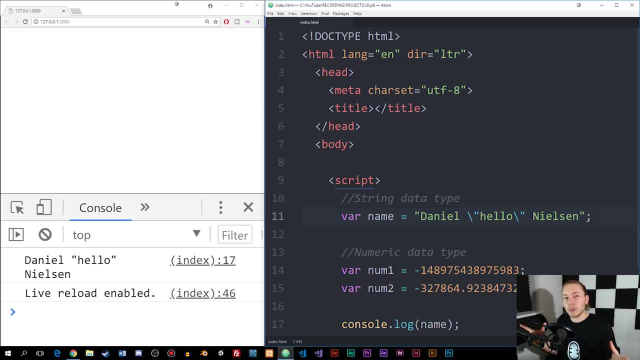 explain when it comes to numeric and string data types, because I might get questions about it in the comments, which is the fact that if I were to create a string data type and just call it something like number instead of equal to a string, and insert some kind of number inside of the string, is this 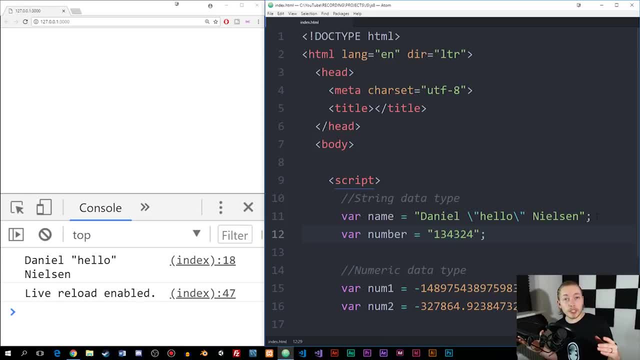 going to be a number data type or is it going to be a string data type? Well, because we wrap double quotes around it, it's going to be a string data type, So this is not going to be seen as it will be seen as a number, but not as a string. 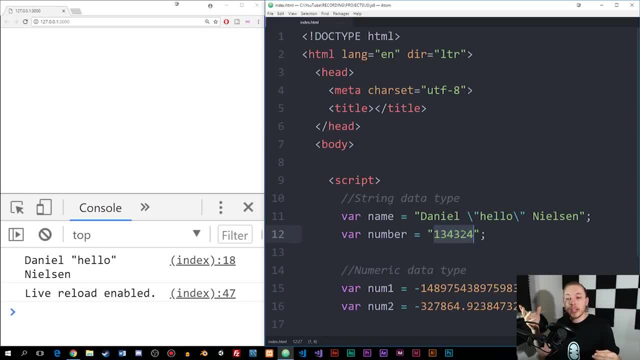 data type. So there's a difference between using numbers and using data types, if you could say that. So this is not going to be a number data type, it's going to be a string data type, because it's inside double quotes. if 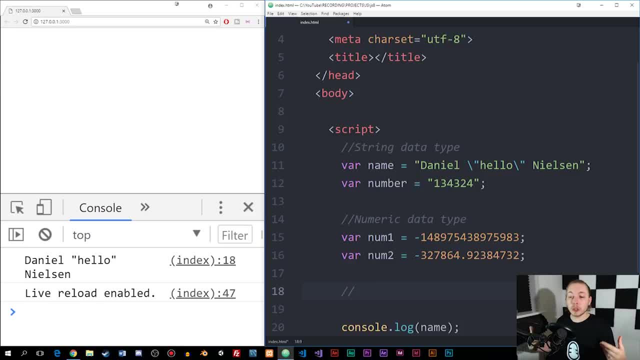 that sort of makes sense. Now, the next type of data I want to talk about is something called a Boolean, Which is something that we also use quite a lot when it comes to using JavaScript, because a Boolean is a true or false statement, And in JavaScript, we 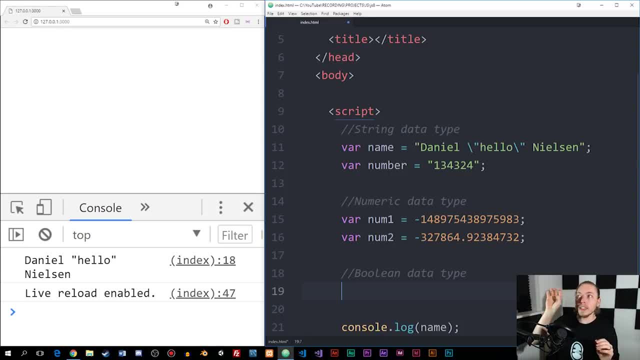 do a lot of things like conditions, which means that we say: is this the same as this over here, or is this statement true or false? then do something inside the code. So we use Booleans a lot when it comes to writing scripts inside. 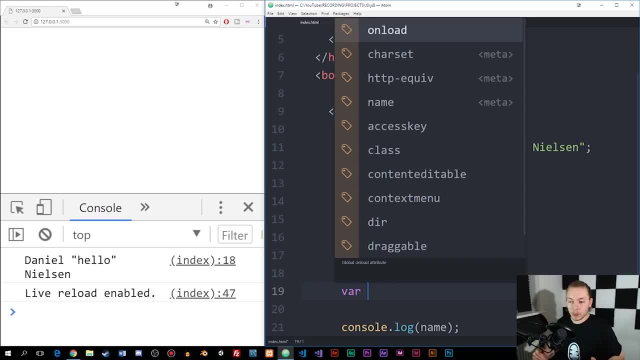 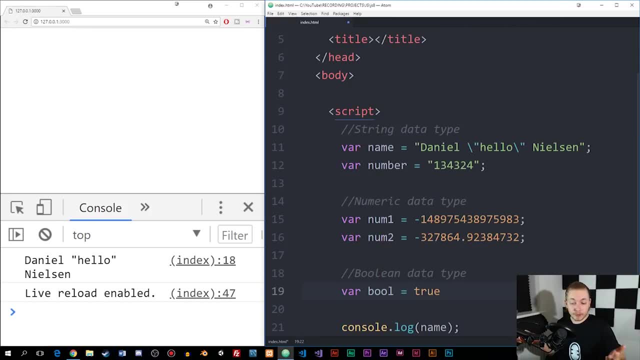 JavaScript, So a Boolean. if I were to just write a variable here, you can just say variable bool, just to give it a name, set it equal to true. or I could create one just going to create a new one, and set it equal to false and we're. 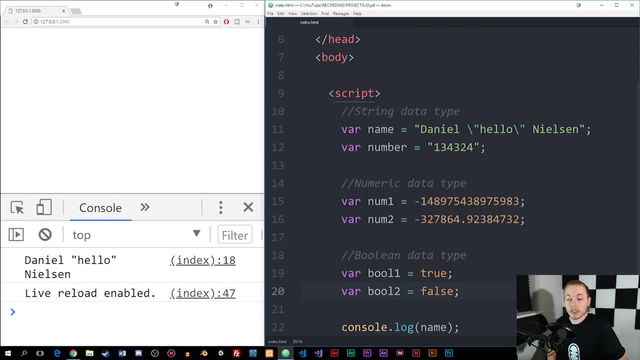 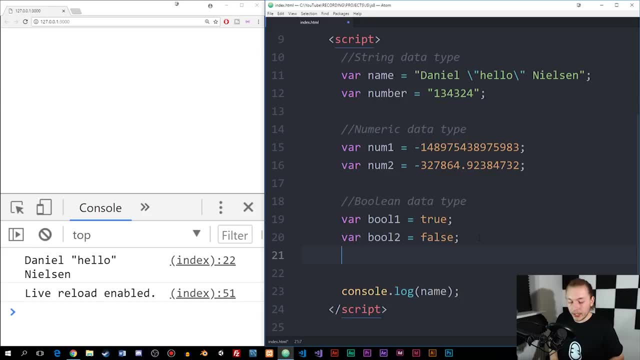 just gonna make sure we don't have the same names for these variables here, like so. Now, when it comes to Booleans inside JavaScript, there's another thing I want to show you, which is that if I were to create a third Boolean down here and call it Boolean, bool3, and set it equal to one, and do some math, and you would see that these variables are called as booleans. 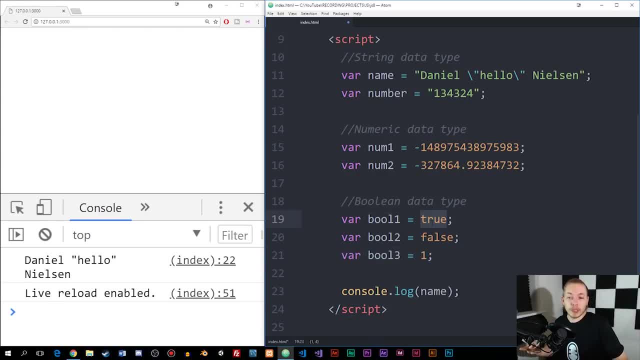 it's going to be the same as setting it equal to true, because in programming one is going to be true and zero is going to be false. so I'm just going to create it here. so the first statement up here is going to be the same thing as down here. 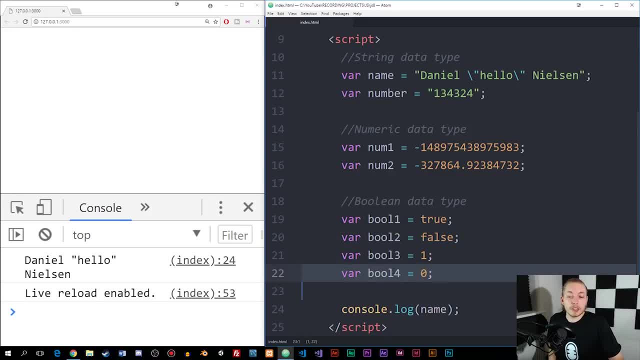 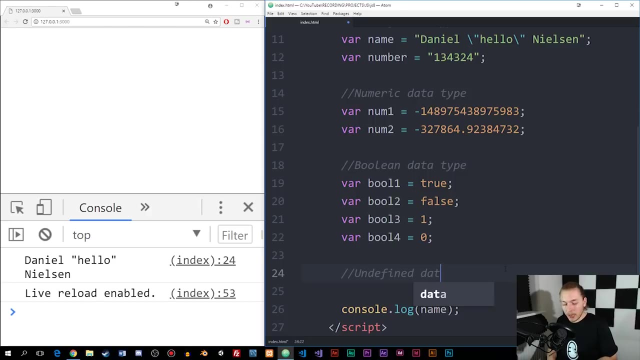 and again, false is going to be the same thing as zero, so, just in case you're aware of it, we can also use ones and zeros to define true and false inside JavaScript. now, the next one I want to talk about is something called undefined, and undefined is something that we did talk about in the previous episode. I do 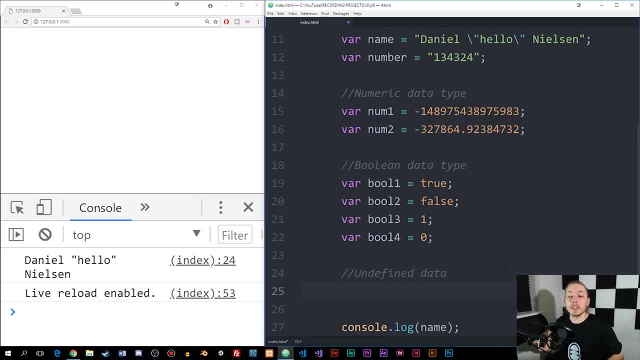 believe, if I remember correctly, and undefined, means that we have a variable that does not have anything set equal to it yet, or we haven't put any data inside the variable. so if we were to go and create a variable and call it something like hey, and just declare it but not set it equal to anything, if I were to take 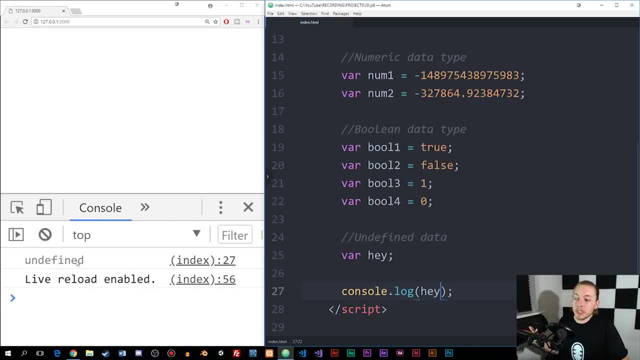 variable head. hey, console lock it. you're going to see that we get undefined, which means that we have no value assigned to this variable. which brings me to the next data type, which is something called null. so we'll just go ahead and create a comment to say we have something called null data type, which is not the same as undefined. 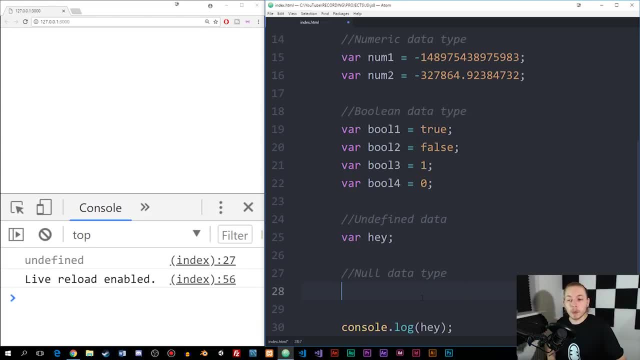 and null data type is when we take a variable and set it equal to nothing. so we do have something that we can use to define that. we have it equal to nothing because we don't want to have undefined inside our variable here. so what I can do is I can say, hey, 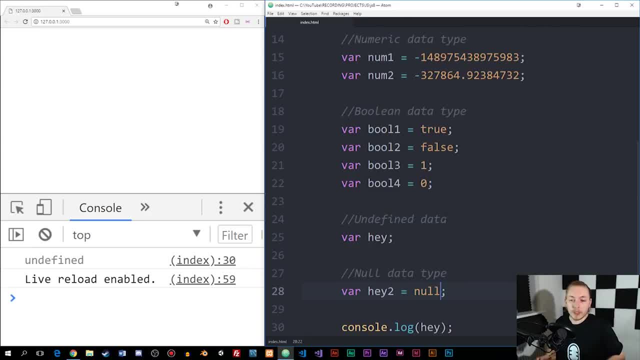 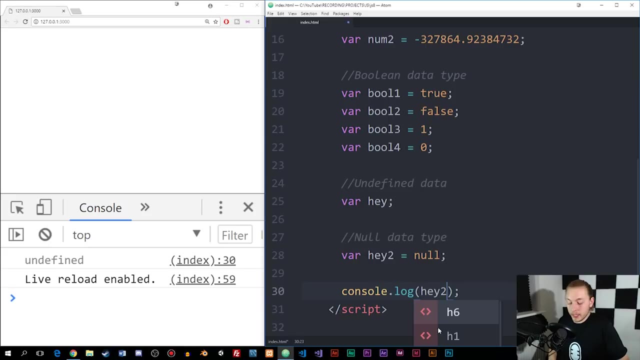 to set it equal to null. which is going to set equal to it's the same thing as saying it's equal to nothing, but undefined says that we haven't set it equal to anything, which is different in JavaScript. so right now, if we were to echo out, hey to, or not echo it out, but console lock it you can. 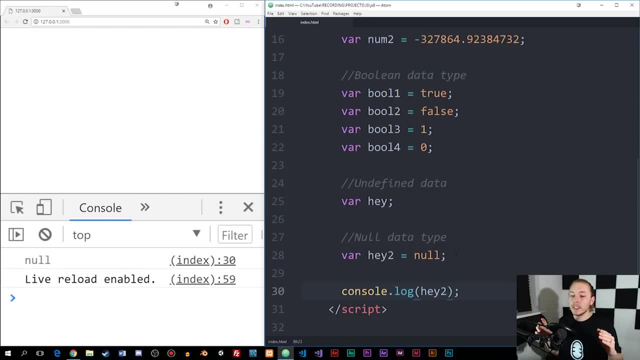 see that we get null inside our browser here now. at the beginning of this episode I mentioned something about JavaScript being able to tell what kind of data inserted inside a variable, but we as humans, if we were to see it inside the browser, might not always be able to tell what kind of data that's inside the 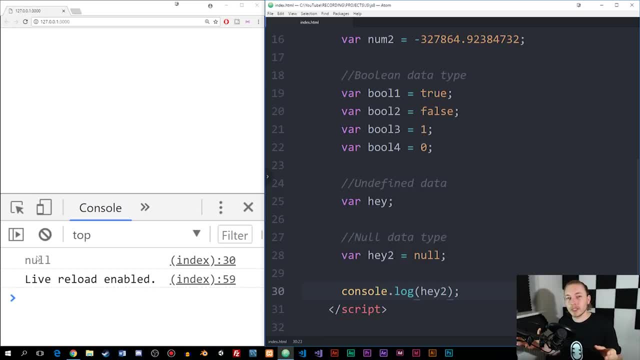 variable. so if you want to actually know what type of data we have inside the variable, we can use something called an operator which is called type of. so if you were to go inside the console Lockdown here and say we have something called type of 445.328.18237.7194.E. 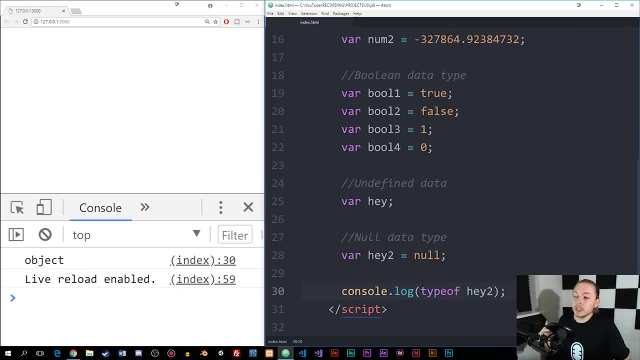 type of space. it's going to go ahead and tell us what kind of object or not, what kind of object. you just just read it inside the browser, so just set it, but what kind of data we have inside the variable. so right now you can actually see that null, it says, is called an object and that is not. 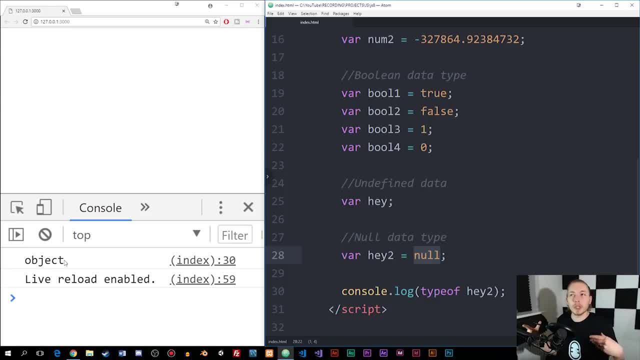 true, but it's something about the browser not being able to tell what exactly null is for a data type, so don't think about the null being an object in this example. here, in all the other data types, it's going to tell us something different, so just ignore the fact that it says object inside. 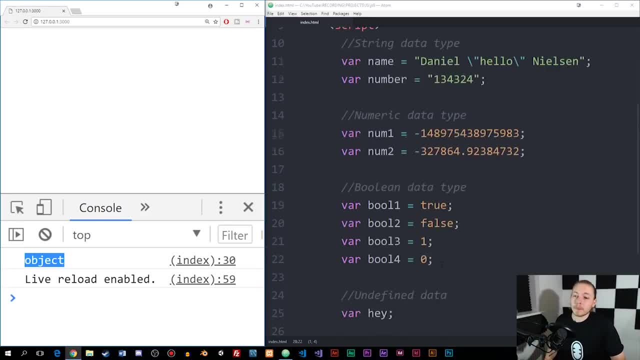 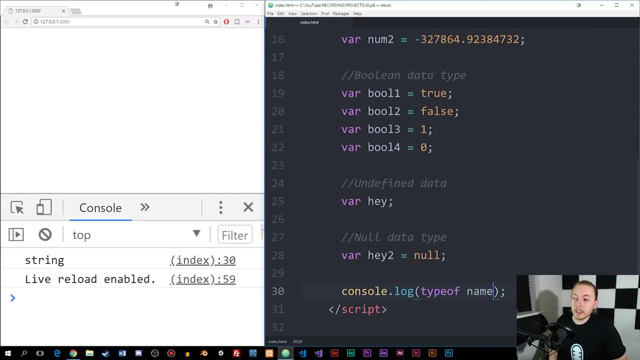 the console because it is a null data type. now if we were to go ahead and use name, which is a string data type, and paste it inside here, you can see it says string inside the browser. if we were to use num1, it's going to see we have a uncalled. 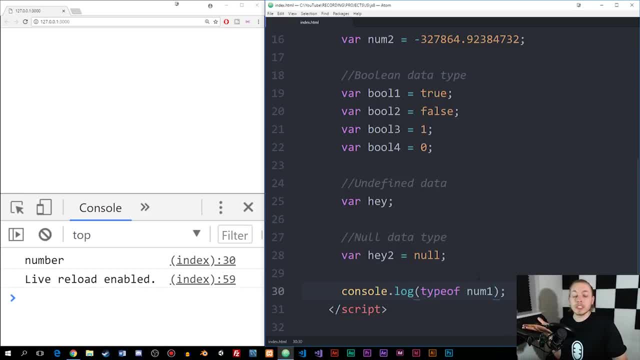 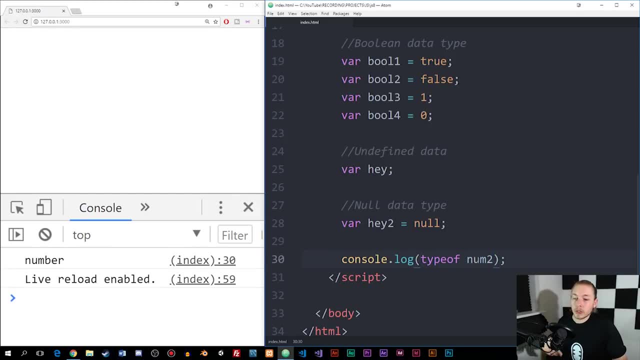 whoops, let's actually insert the right place. it's going to tell us it is a number data type and if we were to use the second number we have up here, which is a integer, it's going to also tell us it's a number, but it is in fact a integer data type, even though it does say number, because 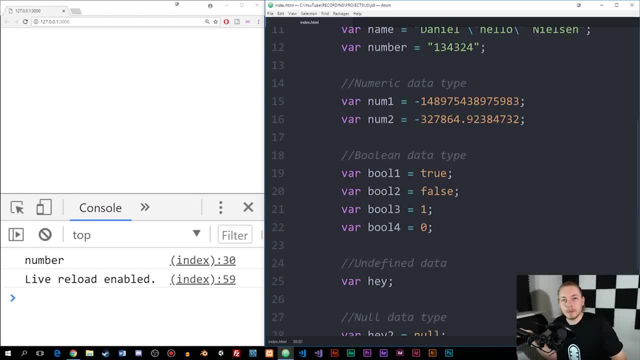 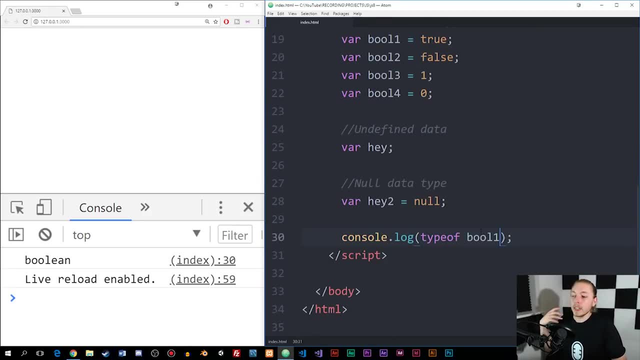 it is essentially a number but it's an integer, if that makes sense. now, if we were to take the next one, called a boolean, and insert it inside the type of save it, you can see we have a boolean. now, if we were to take this one down here, where we set it equal to one, it's going to tell us it's equal to a number because 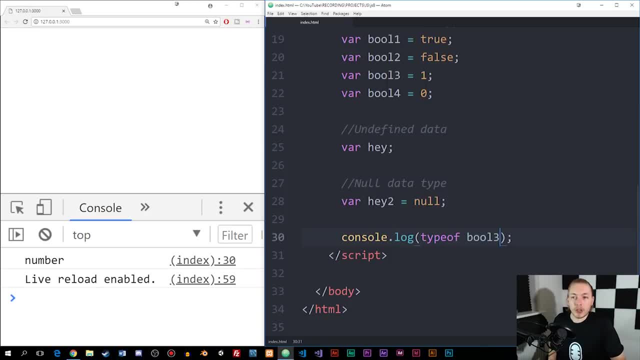 essentially it is a number. it's not going to look at the variable name, just tell it that. oh well, the variable name has bool in it, so it has to be a boolean. it's actually going to go ahead and say it's a number. but if you were to use this in a condition inside javascript- which again we haven't- 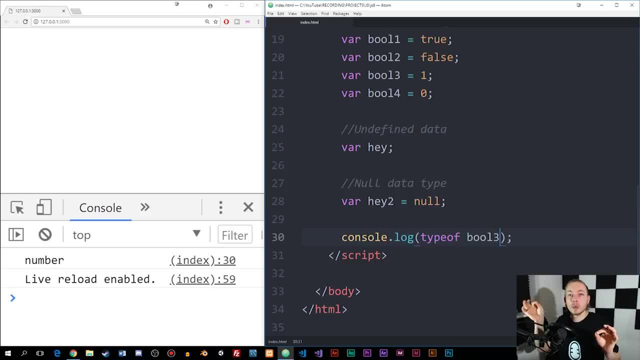 talked about. yet you can use ones and zero to define true and false. so just know that it's still a number data type, but you can use it as a boolean as well. now, if we were to use the variable called hey, you're going to see we get undefined, which we already did inside this example here. so this is: 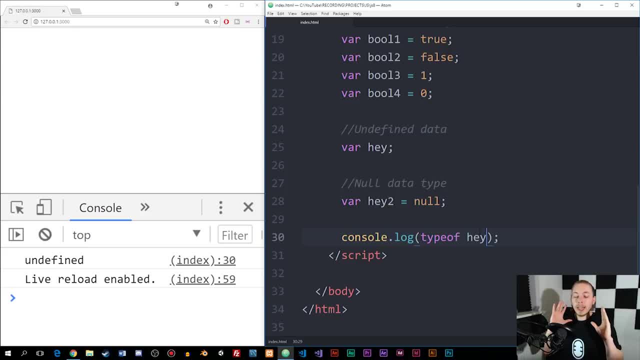 what we have when it comes to data types inside javascript, and these are different types of data. we will be using in the different exercises and you know, scripts that we can write using javascript when we create some different examples, and it's just a good idea to know how to write these sense. 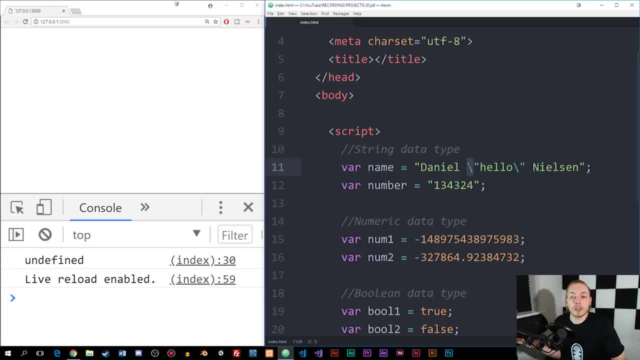 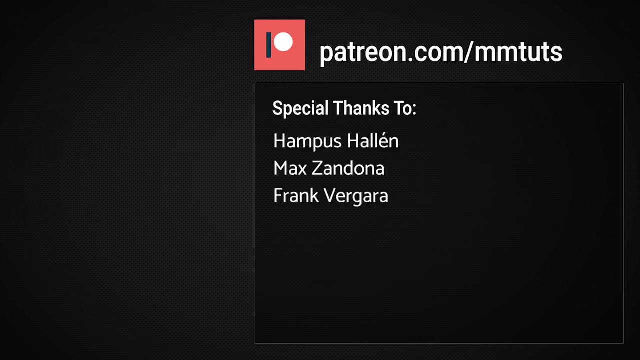 you know, wrapping double quote around string and knowing how to escape characters is a really good thing to know about when it comes to javascript. so i hope you all enjoyed and i'll see you guys next time you.